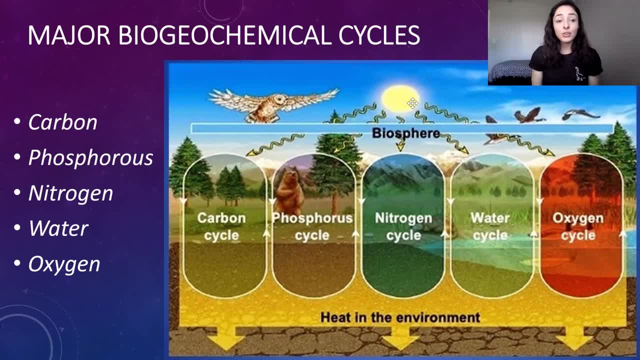 different ways that these chemicals can be cycled through the systems of Earth. Instead, I'm going to be talking mainly about the factors that control biogeochemical cycling on Earth, and to do this, I'm going to be talking mainly about the carbon and oxygen cycles and later in the 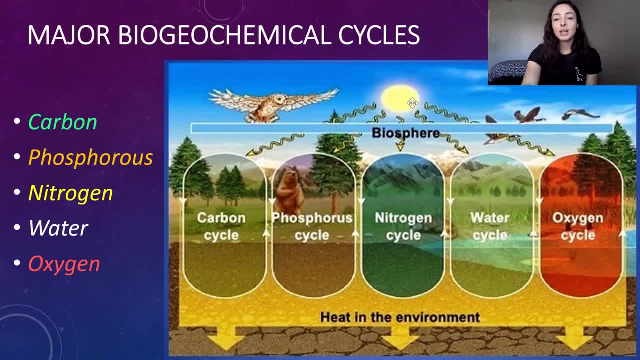 next video, I'm going to talk a little bit about phosphorus and nitrogen, because those are major nutrients that can cause anoxia, which is something we'll talk about next time as well, And then the water cycle is something that, throughout talking about these other cycles, we're basically also 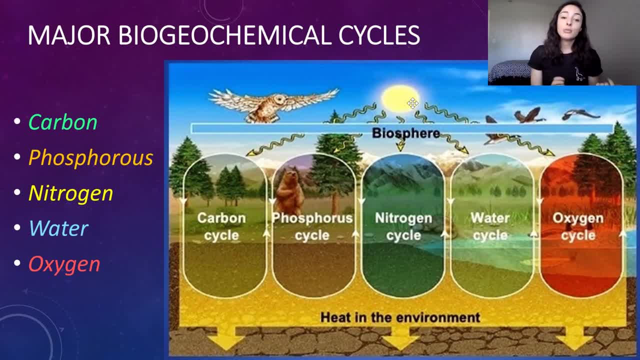 going to be talking about, because the water cycle is a major component of moving all of these other cycles through their cycles, And the reason this is is because water bodies can act as major chemical reservoirs, Bringing us to our next slide: chemical reservoirs. 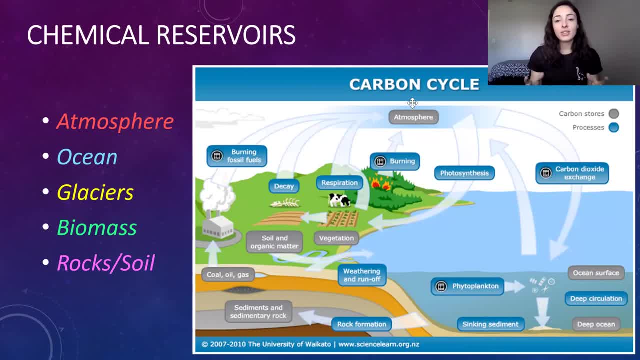 What are they? Well, as we see in the example here to the right, we have the carbon cycle shown and they have this label at the top right called carbon stores. All these gray boxes like atmosphere, ocean surface, ocean, deep ocean, rock, soil, vegetation, all of these gray boxes are chemical. 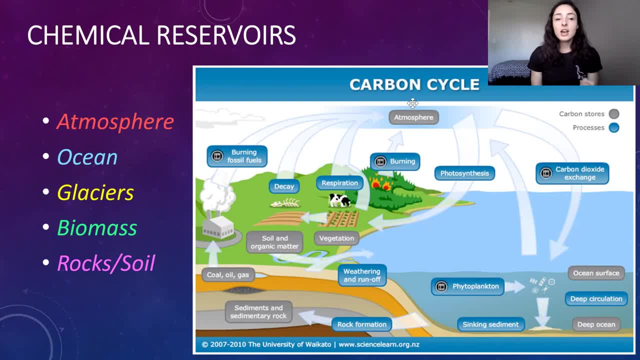 reservoirs and all of the blue boxes are processes. The chemical reservoirs are basically exactly what they sound like. They're like boxes that hold the chemicals. For example, as we talk about carbon dioxide in the atmosphere today, carbon dioxide is the chemical and the atmosphere is 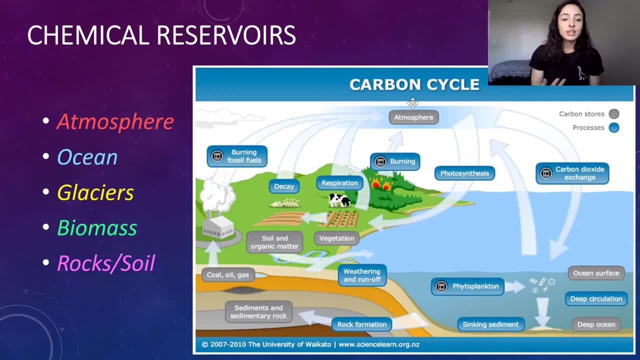 the reservoir for that chemical. Additionally, we have the ocean, glaciers, biomass and rocks and soil. that can also act as chemical reservoirs And as the processes that move around carbon, like respiration, release of carbon dioxide or photosynthesis taking up carbon dioxide, can move. 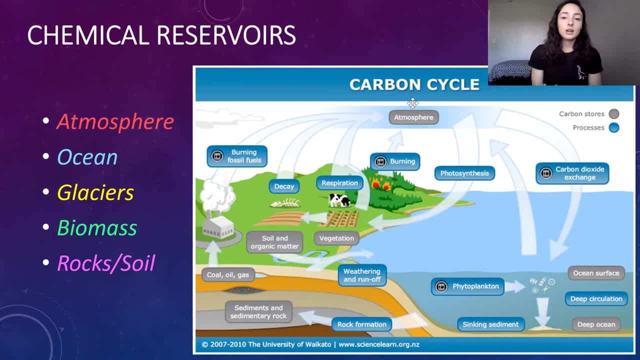 this carbon around. what is happening through those processes is moving the carbon from reservoir to reservoir, And so now that we understand what the major biogeochemical cycles are and how they move between different chemical reservoirs, I want to talk in this video a lot. 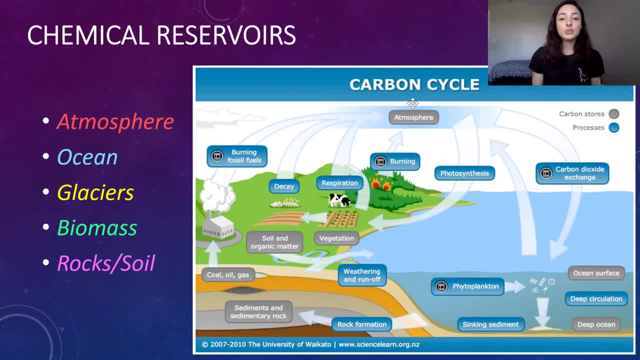 about the photosynthesis and respiration cycle. But to do so we first need to talk a little bit about greenhouse gases, to understand a little bit about why carbon dioxide in the atmosphere is even important, And then we can move on to the rest of the video. So I have here this animation. 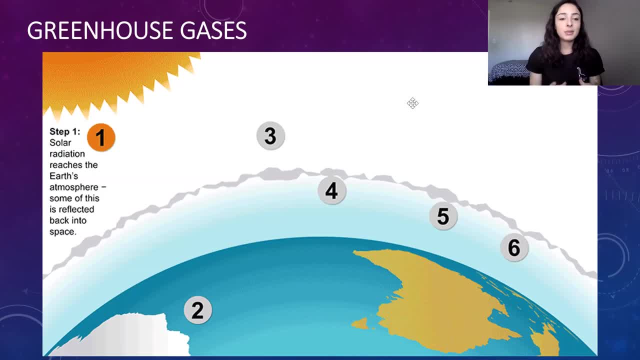 of the greenhouse gas effect. There's numbered steps throughout this animation. First, solar radiation reaches earth's surface and some of that radiation gets reflected back into space. However, some of that radiation gets absorbed by earth's surface. And when it's absorbed, 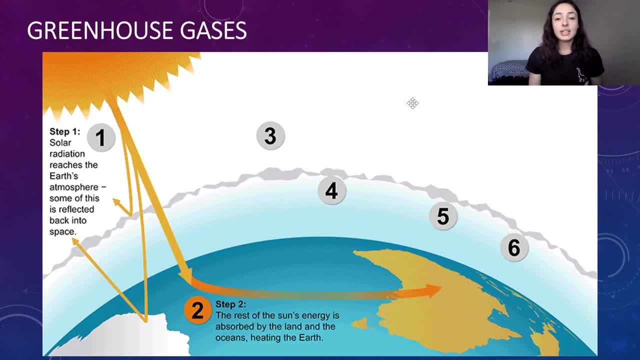 it can move through earth's systems- heating the ocean, heating the land, etc. And then it can be re-radiated back into space. And when heat re-radiates back into space from earth, some of this heat can be re-scattered by carbon dioxide and other greenhouse gases in the atmosphere. 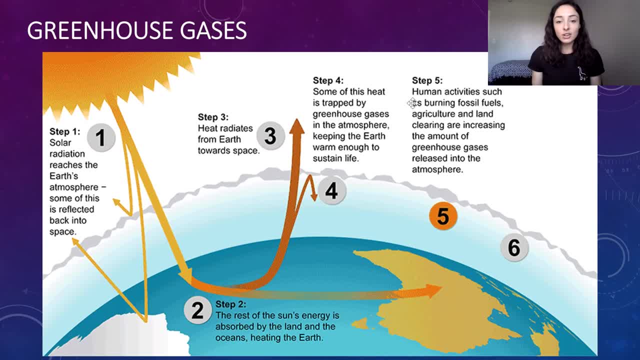 and therefore stay in the atmosphere and continue to heat the earth. This is the greenhouse gas effect And therefore, when the concentration of the greenhouse gas is in the atmosphere, greenhouse gases in the atmosphere increases, the warming of earth increases And in this 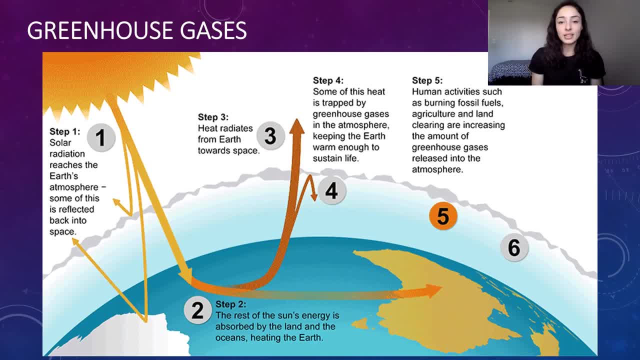 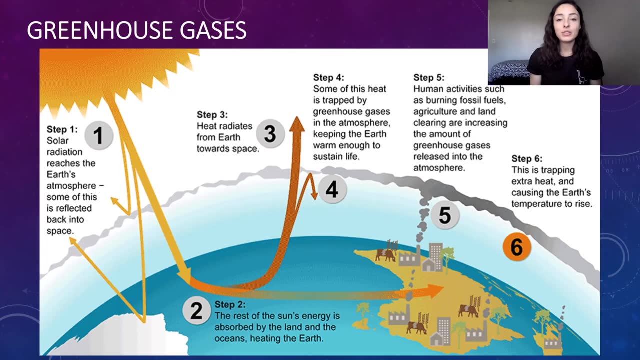 animation. they're showing that as humans increase greenhouse gas concentration in the atmosphere, the global warming situation continues to compound itself and get worse. However, I want to stress that humans are not the only ones that can change or increase or decrease the greenhouse gas concentration in the atmosphere Throughout earth's history. 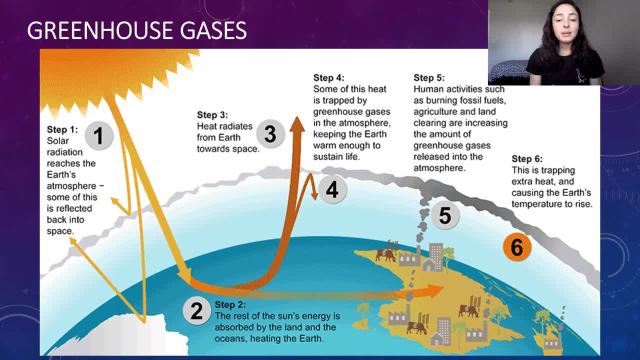 greenhouse gases have increased and decreased in earth's atmosphere many, many times, and the climate has changed, And today we're going to be talking about a lot of the other major factors that can control greenhouse gases in the atmosphere and their movement throughout different chemical reservoirs and how that affects earth's climate as a whole. However, to do so, 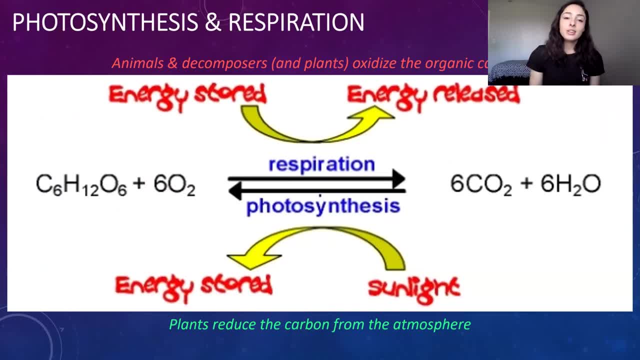 we must talk about the photosynthesis respiration cycle. By understanding the photosynthesis respiration cycle we can understand a little bit better how carbon and oxygen are recycled through our systems. So in this figure we can see that photosynthesis respiration cycle is a. 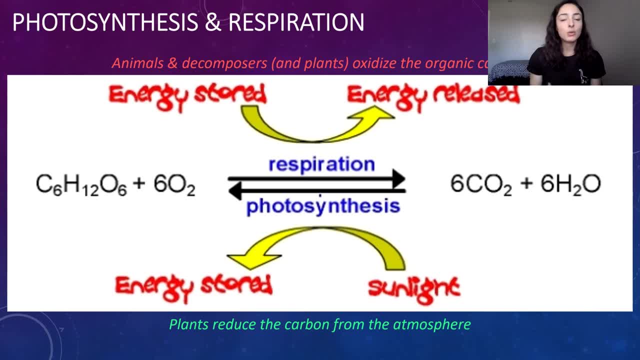 process that takes up carbon dioxide during photosynthesis, and that photosynthesis and respiration are basically the opposite processes from one another. We know that plants take up carbon dioxide during photosynthesis and release oxygen, and we know that we respire by taking up 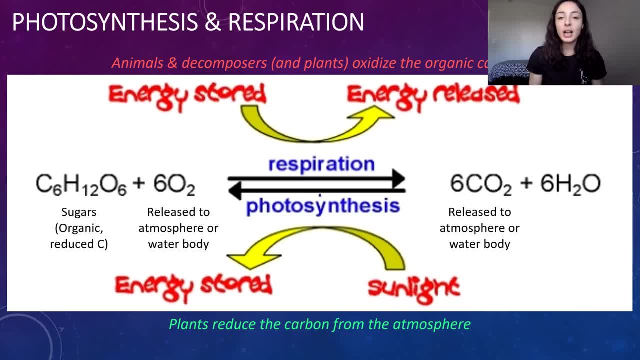 oxygen and releasing carbon dioxide. But to get a little bit more specific here, we can see that what the components of this reaction are are basically sugars or reduced organic carbon- C6H12O6 on the left, and oxygen, which we take up along with sugars to create energy, and then we 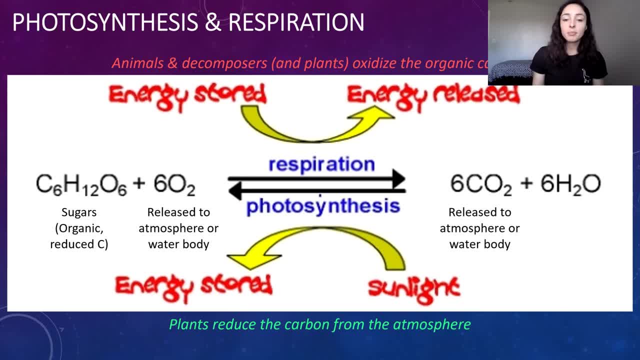 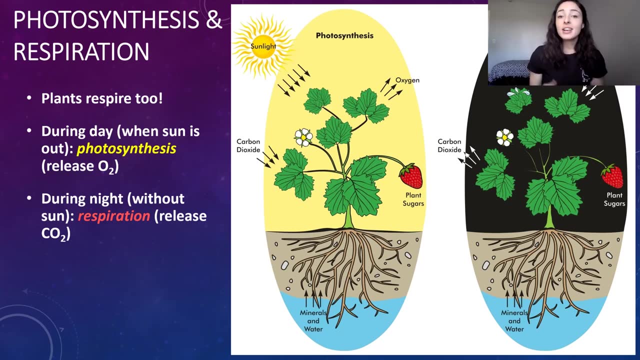 release carbon dioxide. This is the opposite process, in which carbon dioxide and water plus sunlight are used during photosynthesis to create sugars and release oxygen. But something I want to point out here is that plants and all photosynthesizing organisms don't only photosynthesize, they also respire. Yes, 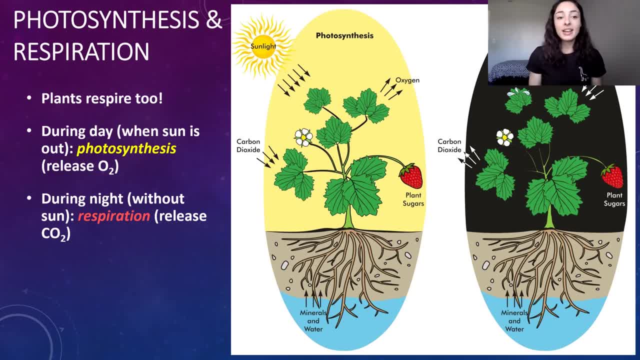 plants take up oxygen and release carbon dioxide at night, and the reason is because the third component of that equation- water, carbon dioxide and sunlight- is only available during the day, And so when sunlight's not available, plants do respire, They release carbon dioxide. And so now you? 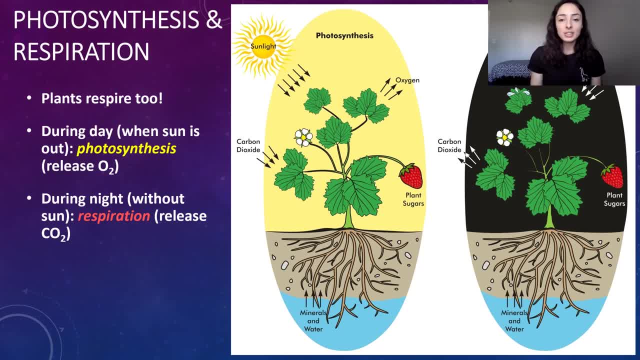 might be thinking that if plants take up carbon during the day and release it during the night, then why do we think that planting more trees will sequester carbon and store that carbon? You might be thinking that it's futile if they're just going to release all their 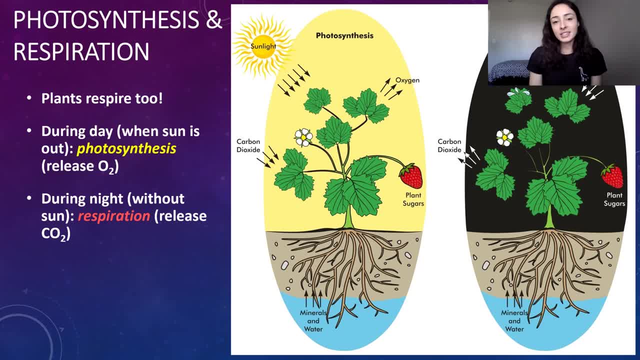 carbon that they took up during the day at night. Well, this isn't necessarily the case. The net effect of plants and other photosynthesizing organisms is the storage of carbon, because what they do is they create sugars, like we showed in the previous equation, and these 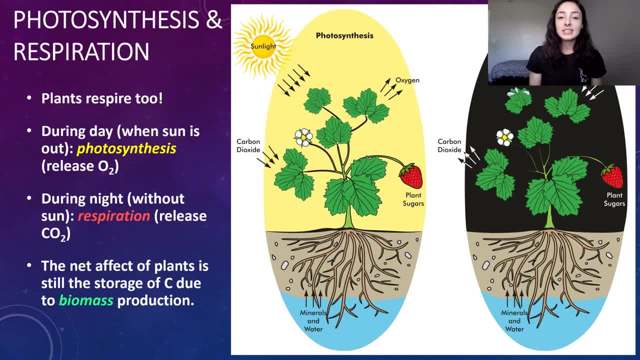 sugars go into building their biomass. The biomass is how plants and other photosynthesizing organisms store carbon, And this production of biomass, which is how plants and trees grow, is the way in which they tip the balance in the favor of storing carbon rather than having a net zero. 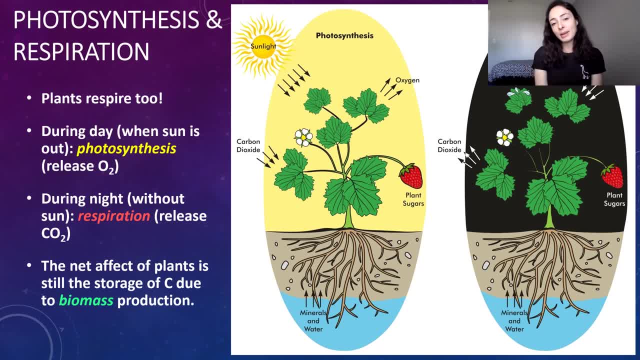 effect on carbon dioxide in the atmosphere. But now the question you might be asking is: well, okay, they store carbon dioxide, but they don't store carbon dioxide in the atmosphere. They store carbon while they're living and growing and they continue to photosynthesize. 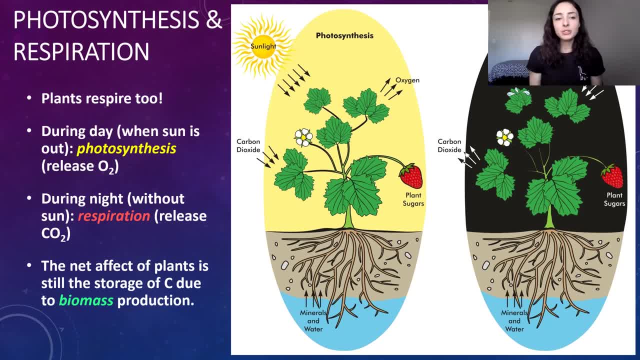 But then what happens when they die? Bacteria and other decomposers just re-oxidize them and the carbon that they stored goes back into the atmosphere as carbon dioxide. Well, yeah, that's true, But not all organic material becomes decomposed and re-oxidized, and 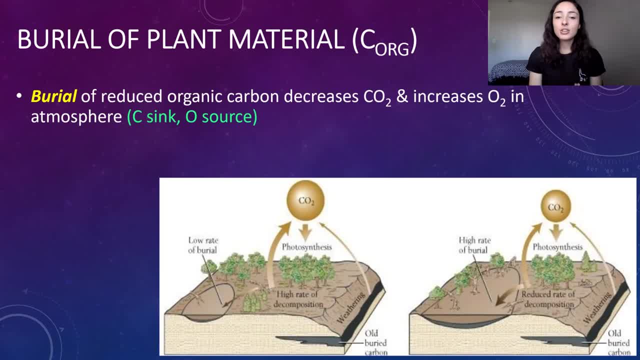 reintroduced into the atmosphere as carbon dioxide. The alternative to decomposition is burial, And because burial prevents reduced organic carbon from becoming oxidized and reintroduced into the atmosphere as carbon dioxide, it's hard to get it back into the atmosphere. This carbon burial acts as a carbon sink and an oxygen source to the atmosphere. Oxygen increases. 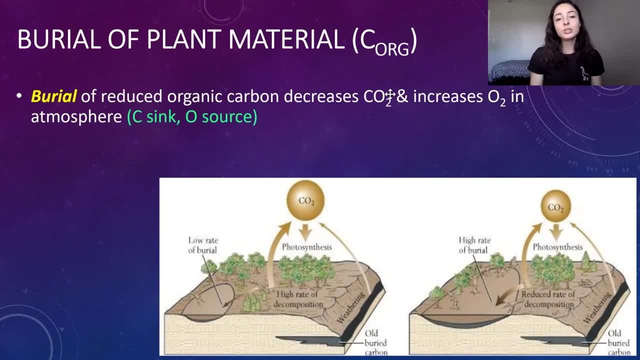 in the atmosphere due to carbon burial, because it's not being used to respire and oxidize that organic material And the carbon is being stored in the rock record for a long period of time. However, decomposition of dead plant material and other organic matter is not the only way. 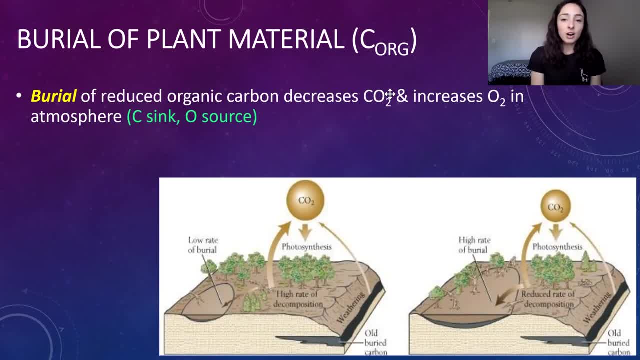 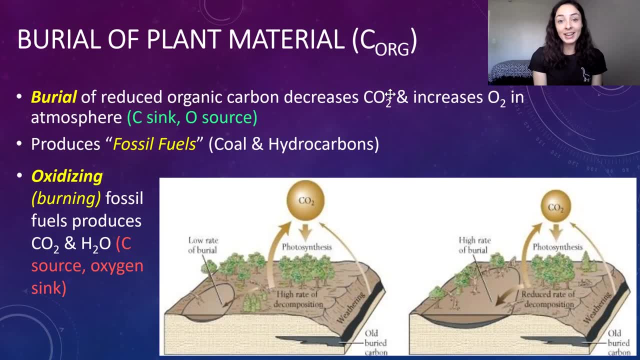 in which carbon dioxide is reintroduced in the atmosphere from stored carbon. In fact, humans invented a whole new way to release carbon dioxide into the atmosphere, And it is way, way faster, Because we are not just using the energy from eating the sugars in trees and 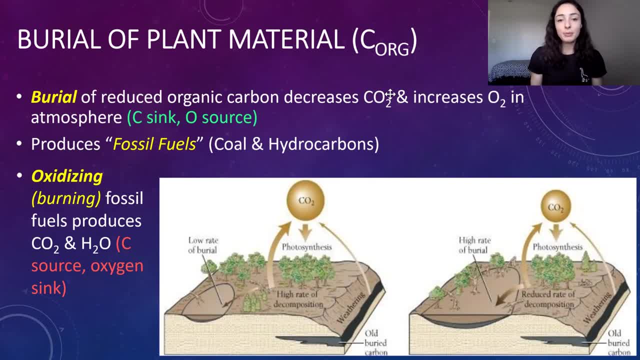 plant material and releasing carbon dioxide from just respiring. we are actually reaching down into the earth, grabbing the buried carbon and directly oxidizing all of that carbon and releasing it back into the atmosphere without it having to wait its millions of years and wait its. 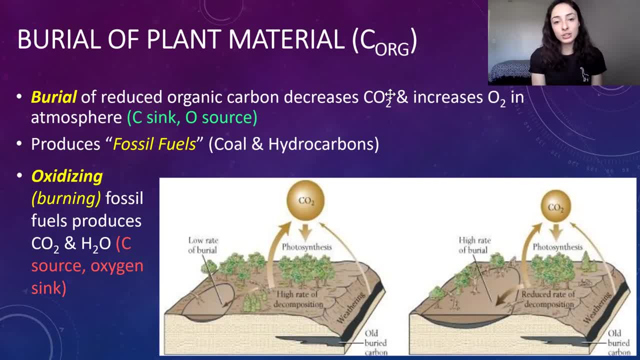 turn for its return to the atmosphere, And that's why carbon dioxide is reintroduced into the atmosphere. And so, because we're expediting the process of oxidizing these buried hydrocarbons or fossil fuels, we are causing a carbon source and an oxygen sink, because it's the opposite process. 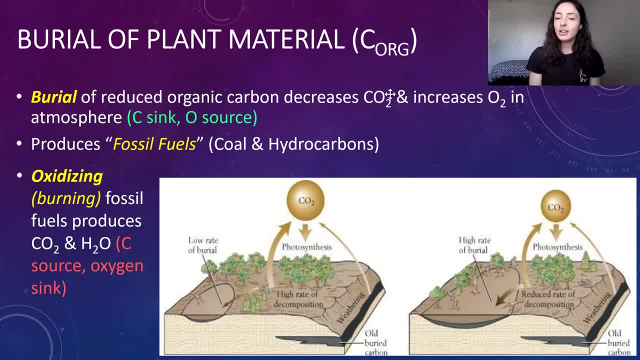 of carbon burial. However, I want to switch gears for a second here, because to understand and track carbon burial events throughout earth's history- and therefore to understand what we're doing to the atmosphere today- necessitates a little bit of understanding of carbon isotopes. 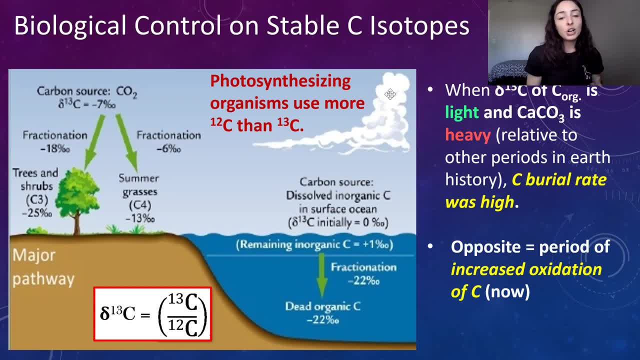 Now, on this slide I'm going to show you a little bit of an example of what we're doing to the atmosphere. So on this slide I show some fractionation patterns of carbon isotopes through natural systems, through the carbon cycle. However, if you're not really familiar with the 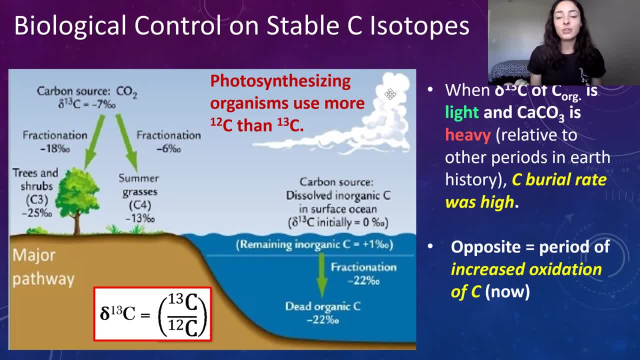 basics of carbon isotopes. I suggest you watch my carbon isotope video before we move on in this video, Because here I'm just going to jump right in to how we can use carbon isotopes to track carbon burial throughout earth's history. Basically, as we see on this slide, we have carbon moving. 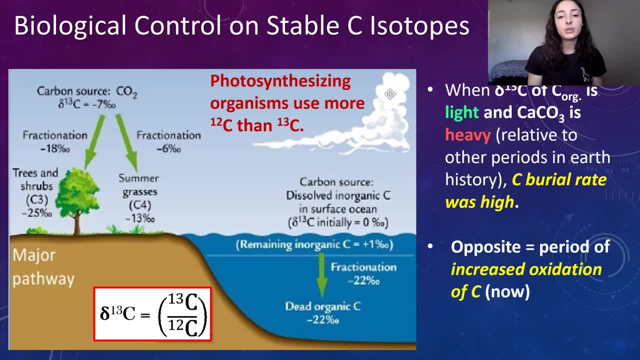 through its chemical reservoirs like the ocean, the atmosphere and organic material in plants and organisms, And as it moves through these chemical reservoirs, the processes that occur to move it between different reservoirs are fractionating the carbon isotopes within the compounds that. 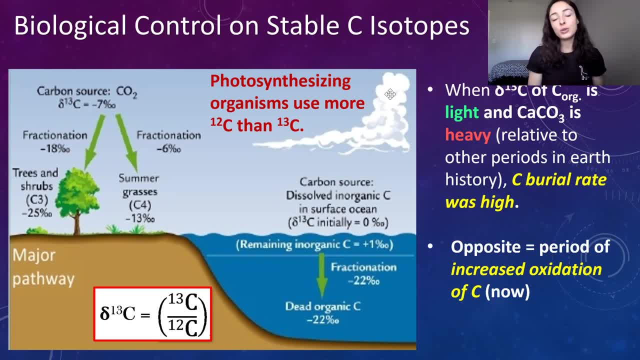 the carbon is incorporated in. An example of this fractionation occurs in photosynthesis. Photosynthesizing organisms take up more carbon-12 or light carbon isotopes than they do heavy carbon-13 isotopes. In doing this, they're fractionating the carbon isotopes. 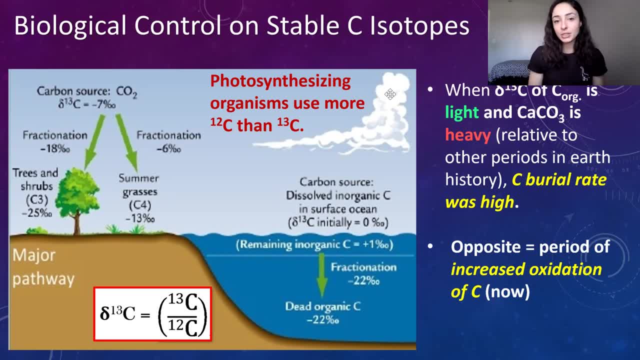 They're incorporating very light carbon isotopes in their organic material. therefore, organic carbon that gets buried has a very light carbon isotope signature and they're leaving behind very heavy carbon isotopes to be incorporated into inorganic carbon like calcium carbonate, minerals, And so when we have this organic carbon and these inorganic 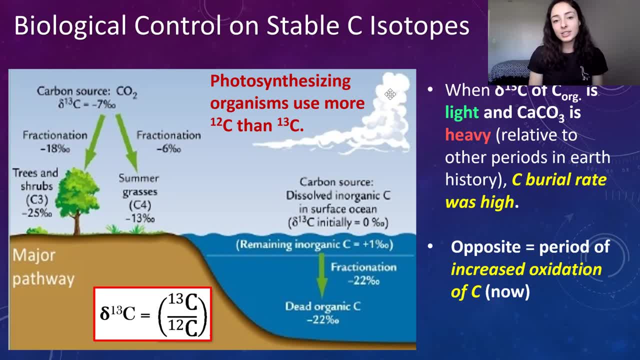 carbon minerals in the rock record, we can measure their isotopes to understand a little bit about the carbon burial rate during the time of their deposition. So, for example, when we have very light organic carbon in the rock record compared to relatively very heavy calcium carbonate minerals. 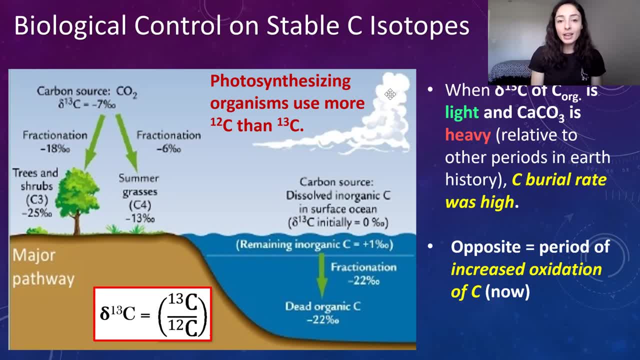 we know the burial rate of carbon was very high because when the organic material from the plants and photosynthesizing organisms that cause that huge fractionation of carbon isotopes gets buried, that leaves behind only very heavy isotopes for calcium carbonate to incorporate in their minerals. 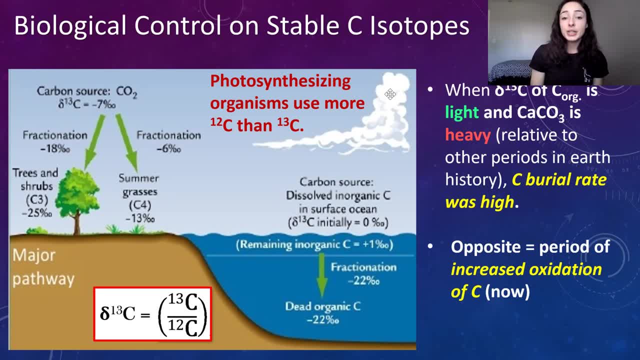 The opposite can be seen in a period of increased oxidation of carbon. So, for example, now we're taking a lot of buried carbon and releasing all those light carbon isotopes into the atmosphere, allowing both organic and inorganic carbon to be incorporated into the rock record. 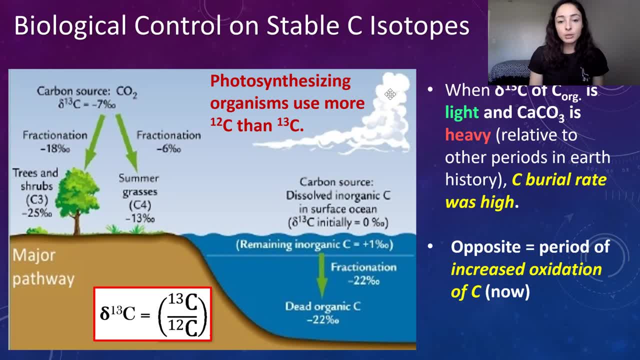 So, for example, when we have very heavy carbon isotopes in the rock record, we can measure very heavy carbon isotopes in the rock record, allowing both organic and inorganic carbon to incorporate light and heavy carbon isotopes into their mineral structures And therefore, 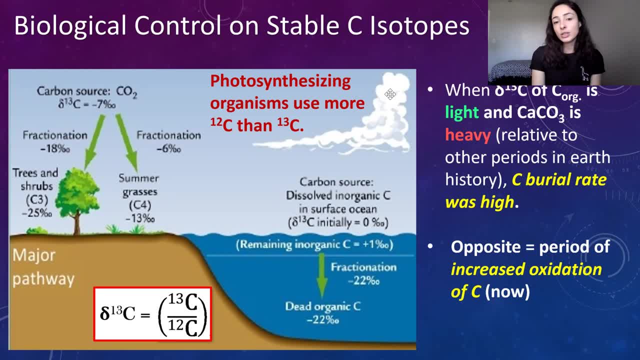 the carbon isotope ratios, or delta C13, of organic carbon compared to that of calcium carbonate during times of decreased carbon burial rate and increased oxidation of organic carbon are going to be relatively similar or less different, less fractionated from one another, because they both 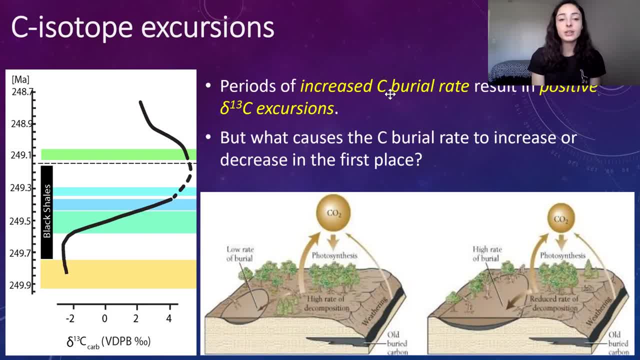 have access to the same light and heavy carbon isotopes. So we can see that the increase in carbon burial rate is shown in the graph to the left here. During this time, around 249 to 248 million years ago, you had this huge jump in carbon isotopes. 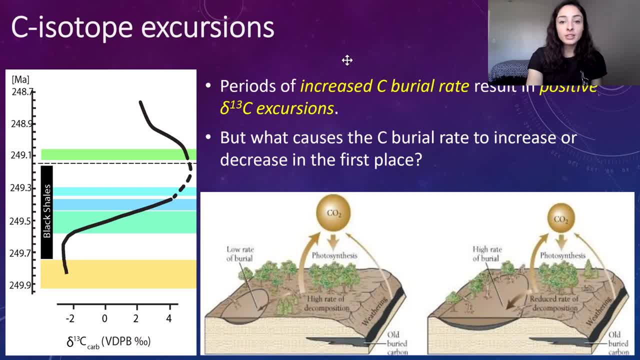 of inorganic carbon or calcium carbonate, which was caused by an increased carbon burial rate during that time. You can see where the black shales were formed due to organic carbon burial, and this left over only very heavy carbon isotopes for calcium carbonate to incorporate. 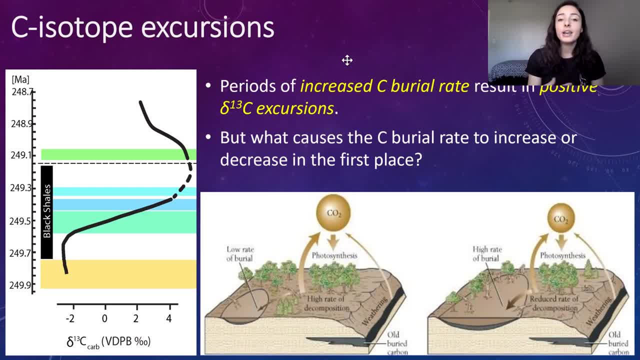 But now that we understand a little bit about why carbon isotopes may become more positive in calcium carbonate during these times, and vice versa when carbon burial rate is low, the question now becomes: what causes carbon burial rate to change in the first place? We know that now we're taking carbon that's buried in the rock. 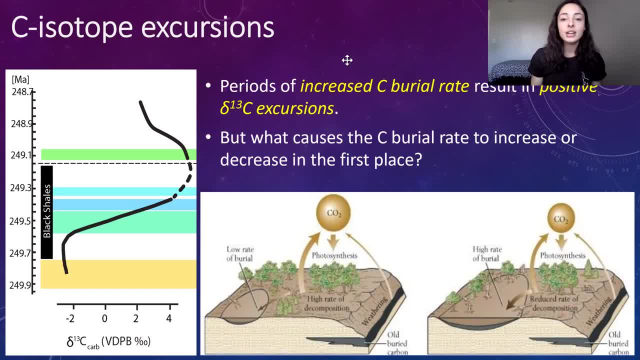 record directly from the rock record and releasing it to the atmosphere and therefore slowing the carbon burial rate directly. But throughout Earth's history, this burial rate has changed many times, including fossil fuel deposits that we have at our disposal today. So what has caused these? 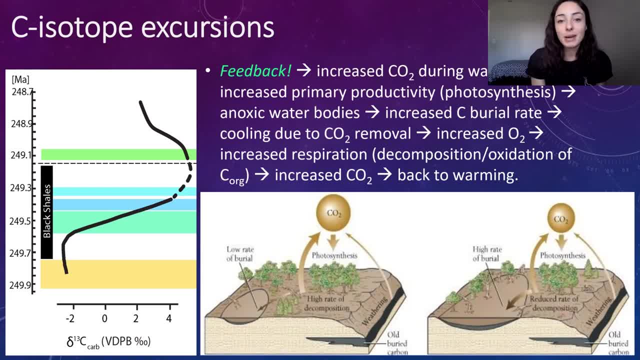 changes throughout Earth's history when we weren't around. The short answer is feedback, but this is a complicated answer and I'm going to explain to you an example of a feedback mechanism right here that is a lot simpler than climate change actually is in real life. So keep in mind. 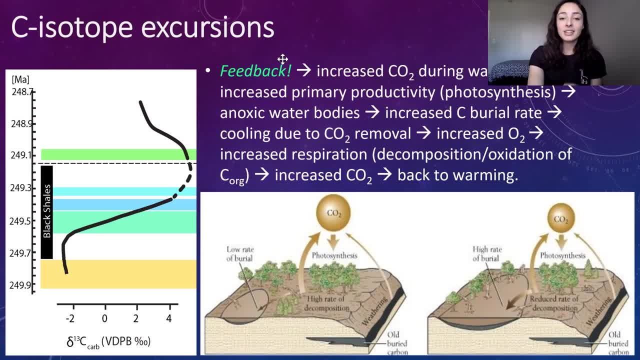 as we go through this example of biogeochemical feedback, that it is not this simple in real life. So I have this example here showing that increased carbon dioxide in the atmosphere causing warming caused increased primary productivity or photosynthesis, and that might cause anoxic water. 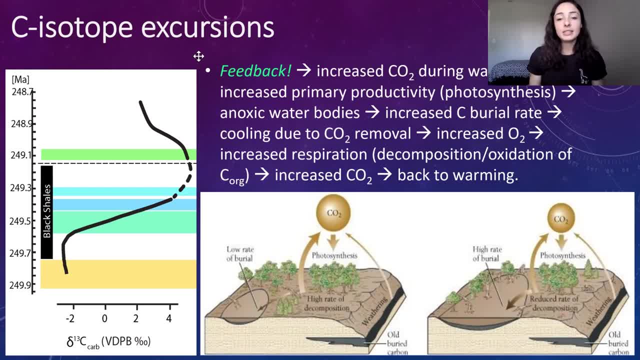 bodies, which we'll talk about in the next video a lot more, but basically this causes an increased carbon burial rate because a lack of oxygen anoxic allows that carbon to be buried without becoming reoxidized first. And this increased carbon burial rate, like we talked about before, 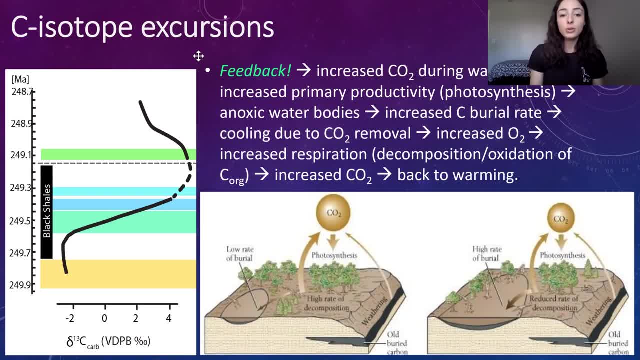 causes a sink of carbon and a source of oxygen, so cooling due to carbon dioxide removal and increased oxygen, which might then cause increased respiration and therefore increased decomposition and oxidation of organic material and therefore increasing carbon dioxide once more, and that causing a return to the warming trend. And so some things I want to. 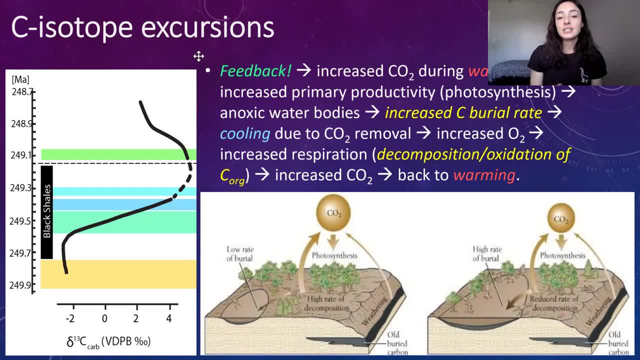 highlight in this feedback mechanism include warming causing something that then causes cooling, and then cooling causing something that then causes warming again. These feedback mechanisms are occurring in loops and they're basically balancing each other out, and this is what's called negative feedback. The negative term in negative feedback is just used to refer to the 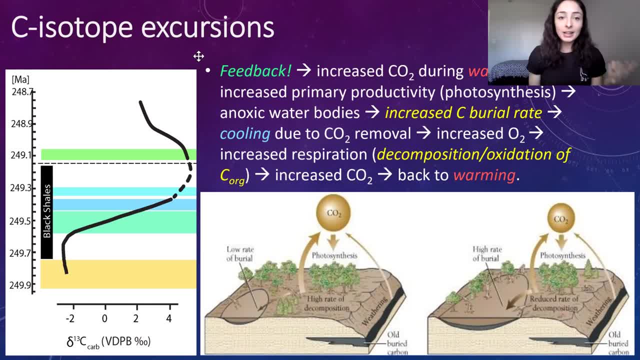 fact that it's a negative feedback. The negative term in negative feedback is just used to refer to that. it's kind of a balancing act. The warming causes something that balances out the warming, causing cooling, and the cooling causes something that balances out the cooling by causing warming. 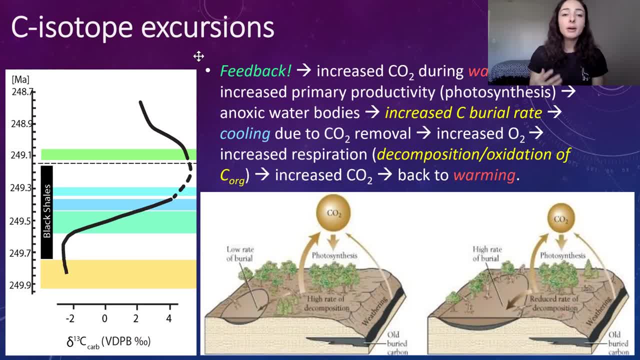 again, and so this balancing effect is negative feedback. However, there are positive feedback mechanisms. I don't have one shown here, but the classic example of a positive feedback mechanism is ice. Ice cover increases surface reflectivity on Earth and therefore, when there's more ice on, 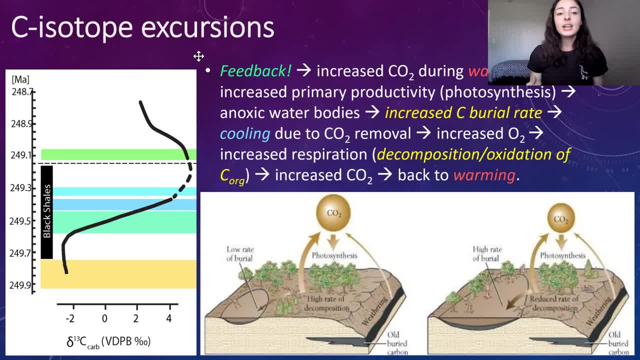 Earth. there's more reflectivity of solar radiation and less heating, causing more cooling, which caused the ice cover to increase in the first place. This compounding effect can go both ways, As warming causes melting of ice. melting of ice causes less surface reflectivity and therefore 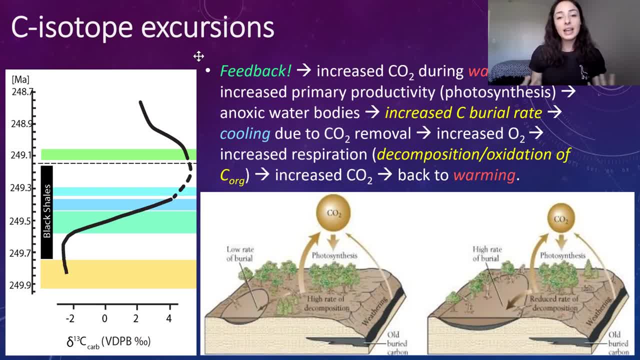 more solar radiation can be absorbed by the increased land area on Earth, and this increased absorption of radiation causes increased warming, and so ice melting compounds the warming effect. and so this is called a positive feedback when, instead of balancing out the system or the trend that is occurring, it just compounds that effect. And so, while this is a positive, 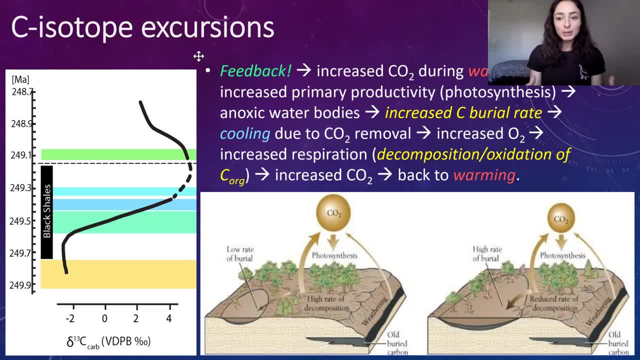 And so these feedback mechanisms are really, really important and I know I'm spending a lot of time on this, but it's super important and I will have later videos that will talk a lot more about feedback, because it can get really complicated. 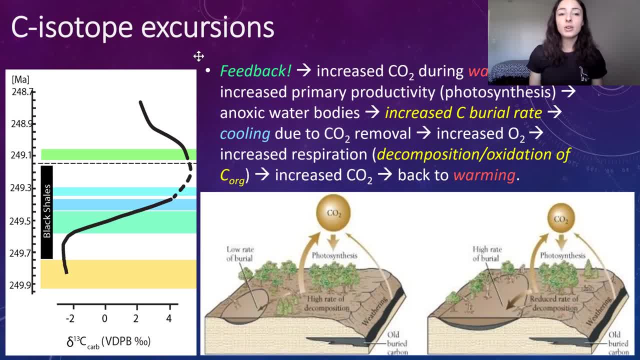 There are a lot of factors that come into this and we'll talk about a lot more of those factors in the next video, as we talk more about feedback in the next video. But for this video I want to finish up with two major uses of carbon isotopes that I think really point out the diversity of this carbon isotope tool and how we can use it to tell so many different things in science in general. 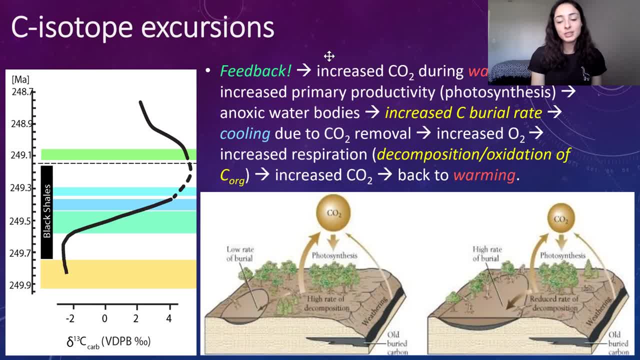 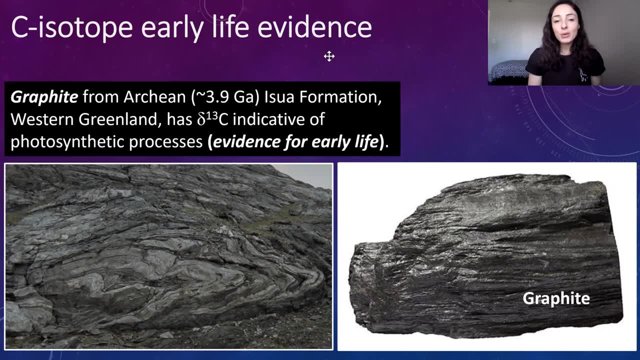 So let's get into these two major uses of carbon isotopes. The first major use I want to point out is the use of carbon isotopes to detect early life on Earth. You might be wondering how the heck does carbon burial rate have anything to do with detecting early life on Earth? 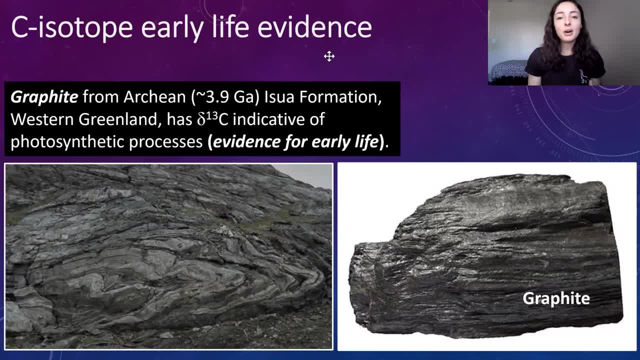 Yes, carbon isotopes. Carbon isotopes aren't fossils per se, but they are biochemical signatures that can act as fossils. The carbon burial rate, as we saw earlier, affected the carbon isotope composition of organic carbon and inorganic carbon in the rock record. 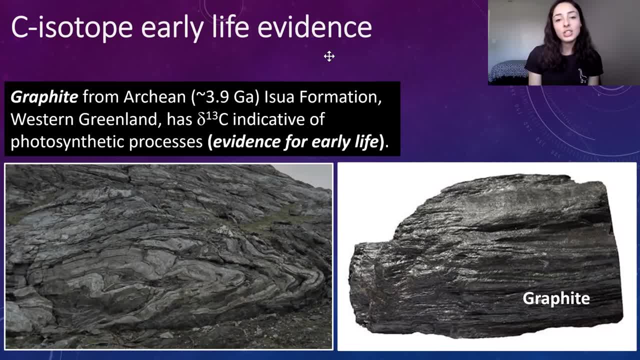 was caused mainly by photosynthesizing organisms fractionating carbon isotopes and taking up very light isotopes of carbon. This really light isotopic signature of organic carbon in the rock record can be traced all the way back to rocks in the Ischua Formation of western Greenland. 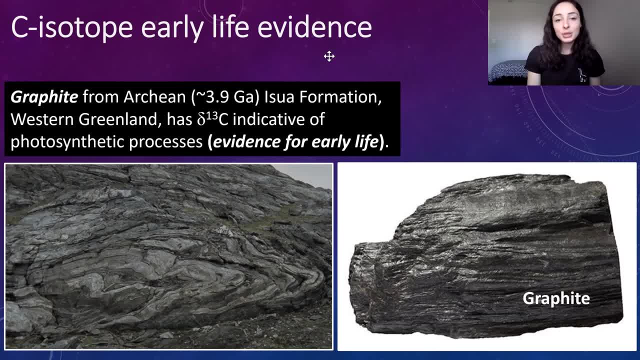 that are overgrown irgendwann With iron and iron. iron in the rock record can kind of suck, because we also cannot corroborate this evidence with other tastes on Earth, or at least that we haven't found yet. It's that we can't corroborate ingredients on Earth anymore, as early in the world of Earth asべ. 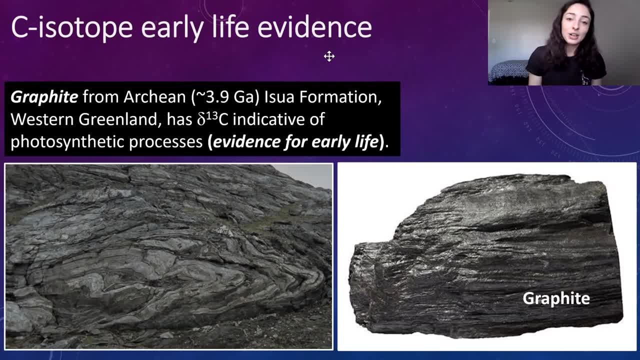 you лうс emм y ren t спасLu أre years ago is a heck of a gnarly start for photosynthesizing organisms on Earth. But again, it's really hard to prove without other rocks from this period that show similar signs, And it's hard. 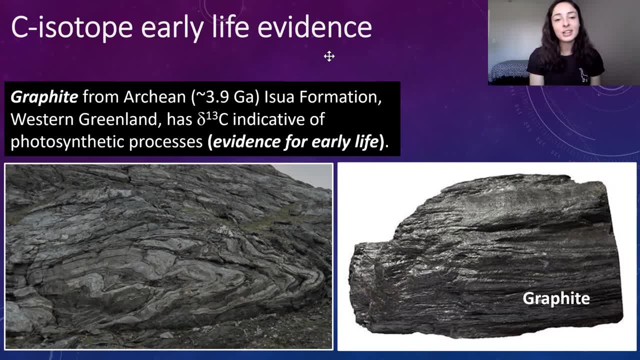 to find those rocks because, again, like we've discussed throughout this entire lecture, things on Earth are typically cyclic and the rock cycle is no exception to that. The rock cycle is a cycle and it recycles rock material And because of this, we have very few rocks that survive this long. 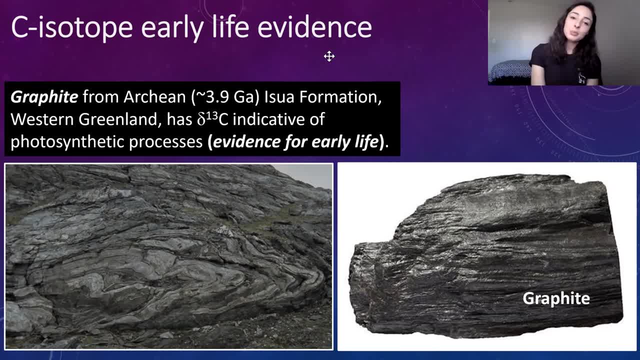 and retain their geochemical signatures. However, I still think it's pretty cool use of carbon isotopes, and one that's worth pointing out, especially because carbon isotopes not only can tell us maybe a little bit about early life on Earth, but can maybe even tell us about the 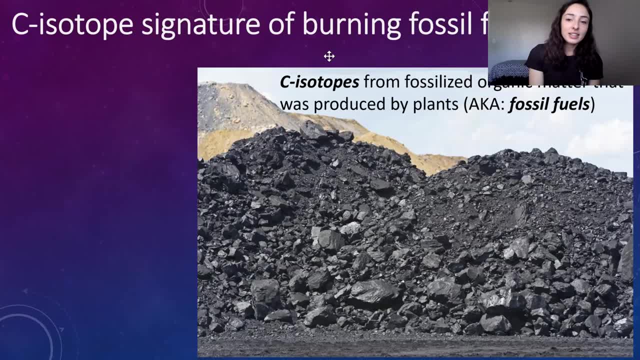 presence of life on other worlds. The last thing I want to discuss is fossil fuels. We talked about carbon isotope signatures being really light in fossil fuels, because the material that makes up fossil fuels is organic carbon material that has preferentially taken up carbon-12 or light carbon. 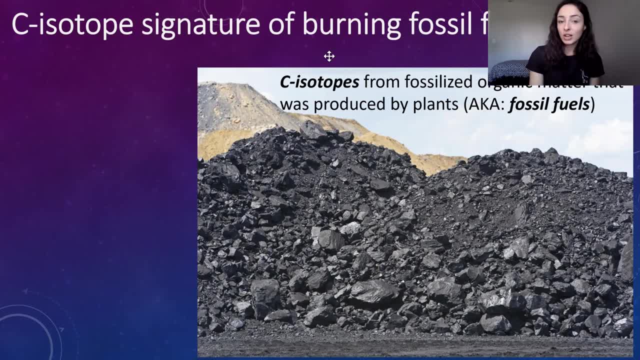 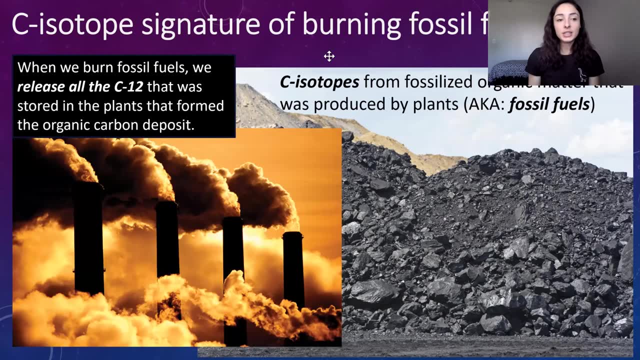 into It's structured And because we then come and use these fossil fuels and burn them and release the carbon from these fossil fuels into the atmosphere as carbon dioxide. we are then releasing all this carbon-12, this light carbon that was stored in these fossil fuels, into the atmosphere, which has 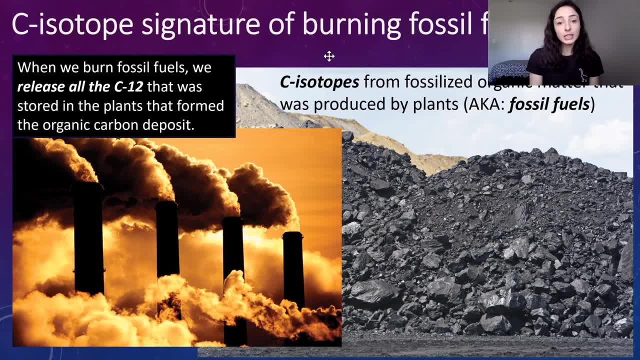 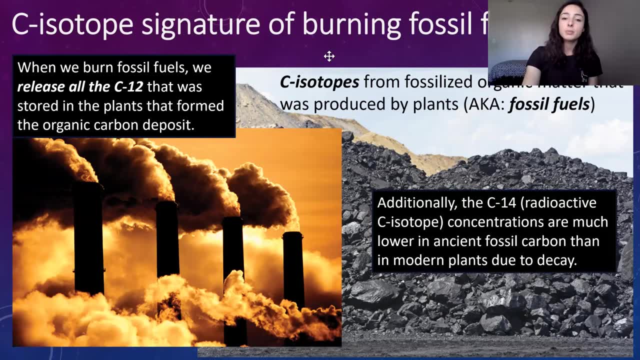 a very different carbon isotope composition than what we're releasing, because what we're releasing has been heavily fractionated. Additionally, the signature of carbon isotopes in organic material or fossil fuels becomes even more specific and distinct from the background carbon in the atmosphere, because what we're releasing has not only a distinct